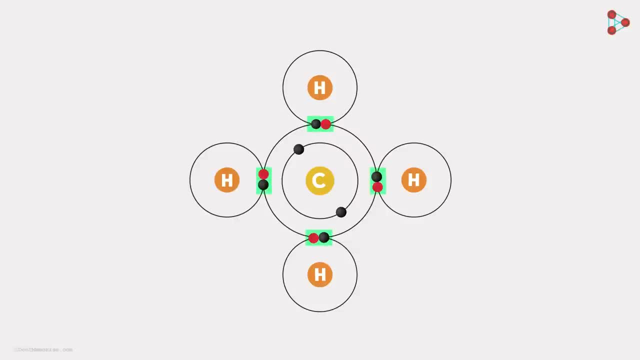 each hydrogen atom attains stability by having two electrons in its shell, and even carbon gets eight electrons in the outermost shell, How One electron from each hydrogen atom makes four, and there are already four valence electrons with carbon. These sum up to attain. 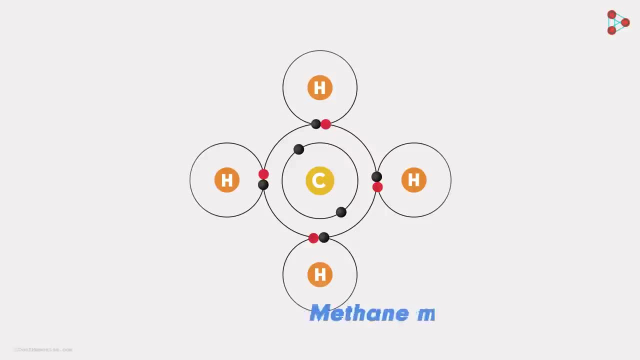 the octet state. This is how methane molecule is formed: A single carbon atom bonded with four hydrogen atoms. Each bond here is a single covalent bond. This is how single covalent bond formation between carbono and any other element looks like You could find it in an energy science. 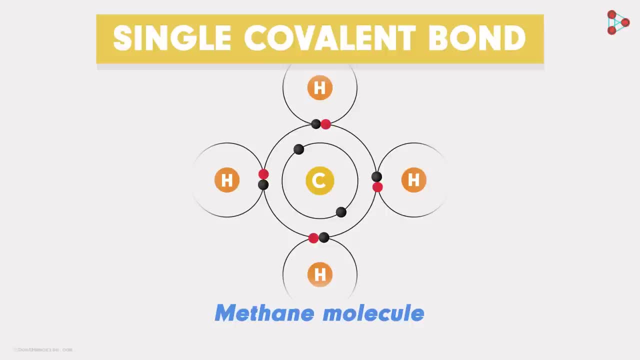 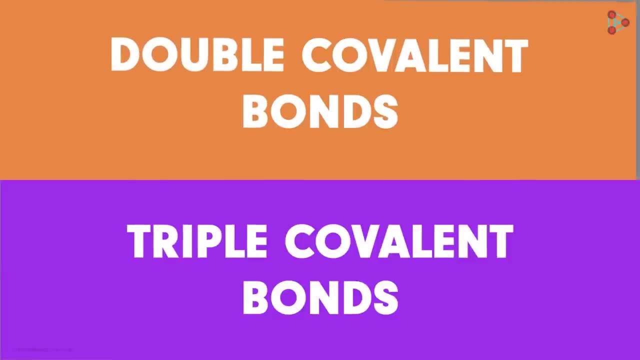 any monovalent element takes place. Now let's talk about the double and the triple covalent bonds formed by carbon. To understand this, we take a simple example of the compound carbon dioxide. Can you draw the typical molecular structure of carbon dioxide? 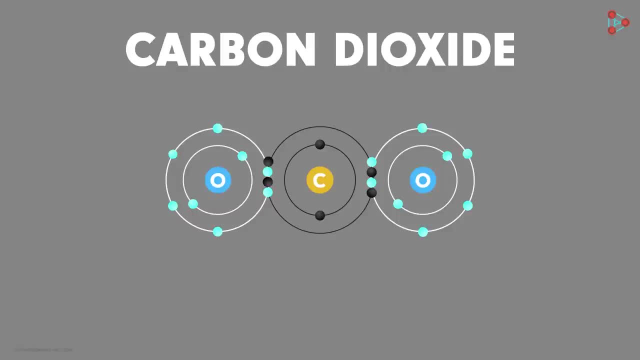 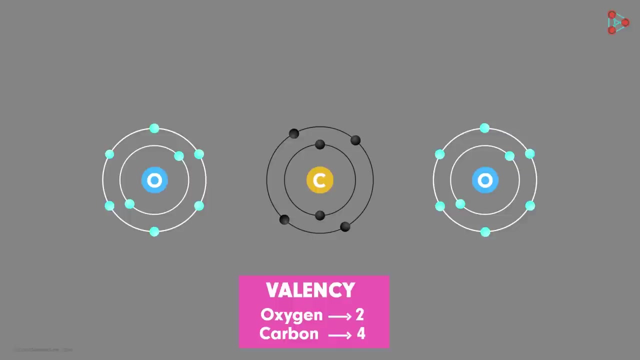 Yes, it appears somewhat like this: Two oxygen atoms bonded with one carbon atom. How is this bond formed? by the way, We know that the valency of oxygen is two, while that of carbon is four. That means, out of the four valence electrons, two electrons will be shared with one oxygen. 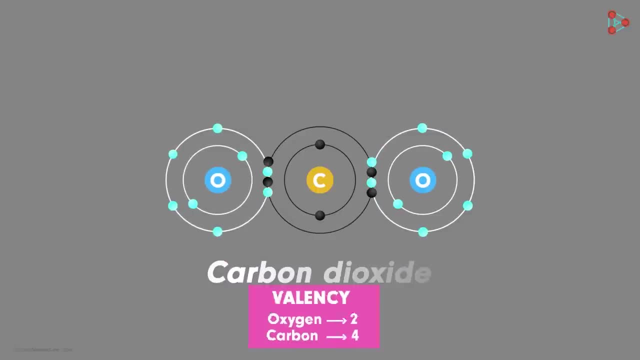 atom, while the remaining two with the second oxygen atom. But sharing means both the atoms will participate in the bond formation right. That is why, at the same time, each oxygen atom also shares two electrons with carbon atom. Such type of sharing enables the atoms to attain stability. 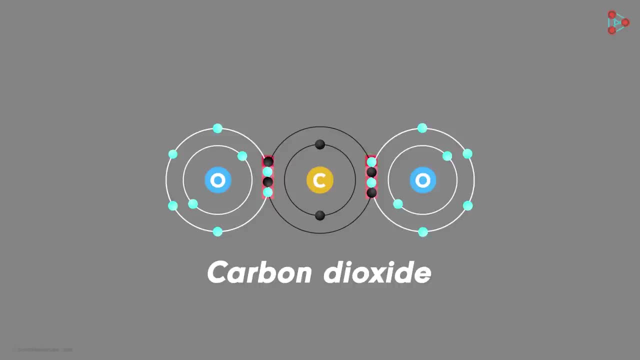 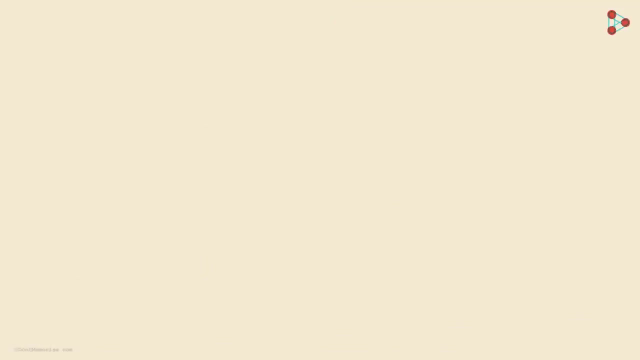 Wait a second. Did you notice that there are four electrons, or simply two pairs of electrons, shared between each oxygen and carbon atom? Yes, That makes it a double covalent bond. right, Absolutely Now. lastly, we take the example of a triple covalent interaction of carbon. 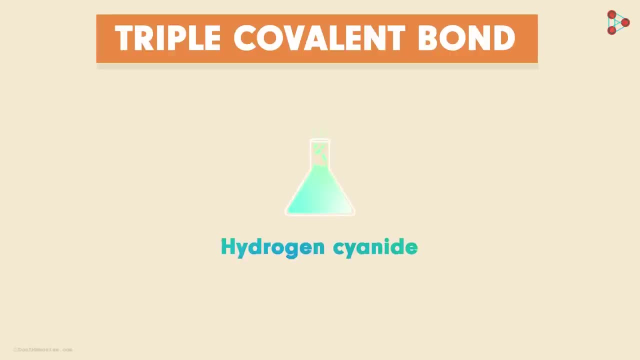 Have you ever come across the compound hydrogen cyanide? Yes, It is an extremely poisonous liquid used for experiments in laboratories. Yes, Do you know what its chemical composition is? It is HCN. So do you know what the structure looks like?